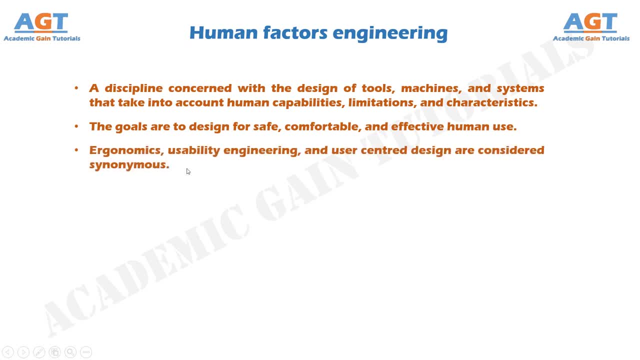 Ergonomics, usability engineering and user-centered design are considered synonymous. Human factors engineering is based on design-related aspects of several biomedical disciplines, including anthropometrics, biomechanics, sensation and perception, anatomy and physiology and cognitive psychology. 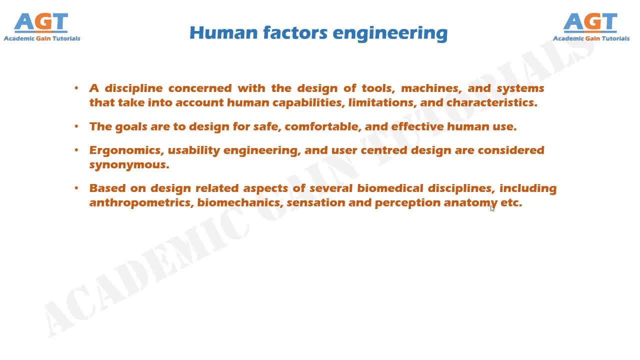 which covers models and theories of human behavior, Human performance, memory and attention. With few exceptions, all machines are designed to be used by humans. Even robots must be programmed by a human. Human factors. engineering is the study of the human-machine interaction and is defined as an applied science that coordinates the design of devices, systems and physical working conditions with the capacities and requirements of the worker. 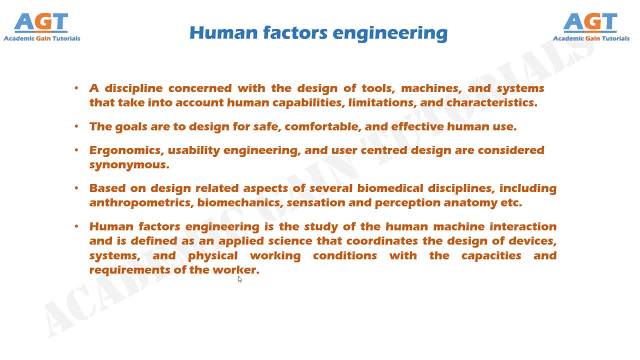 The machine designer must be aware of this. The machine designer must be aware of the subject and design devices to fit the man, rather than expect the man to adapt to fit the machine. The term ergonomics is synonymous with human factors, engineering. 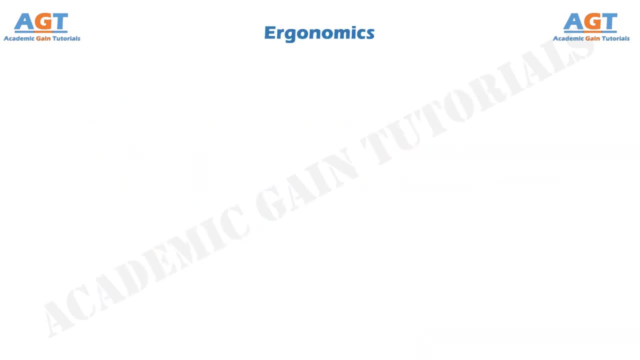 Now let's move into the concept of ergonomics. Ergonomics is the study of the interaction between people and machines and the factors that affect the interaction. Its purpose is to improve the performance of the system by improving human-machine interaction. 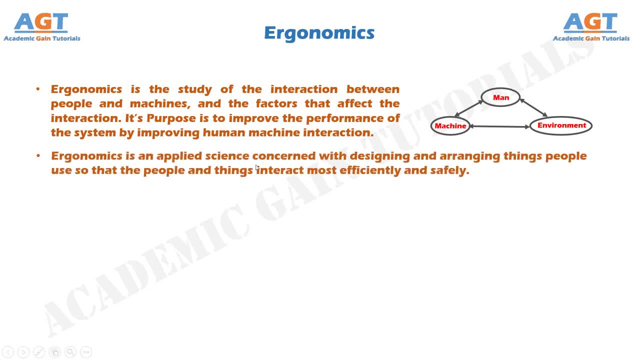 In other words, ergonomics is an applied science concerned with designing and arranging things people use so that the people and things interact most efficiently and safely. So it is also called human engineering or human factors engineering. 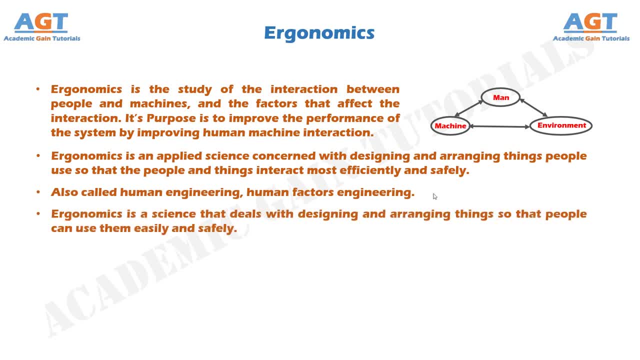 Ergonomics is also defined as a science that deals with designing and arranging things so that people can use them easily and safely. If defined medically, Ergonomics is a scientific discipline which is concerned with improving the productivity, health, safety and comfort of people, as well as promoting effective interaction among people, technology and the environment. 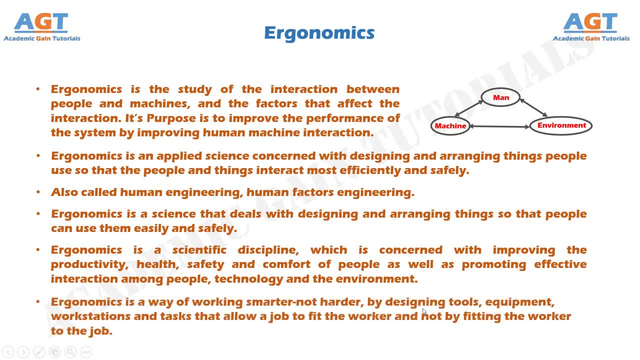 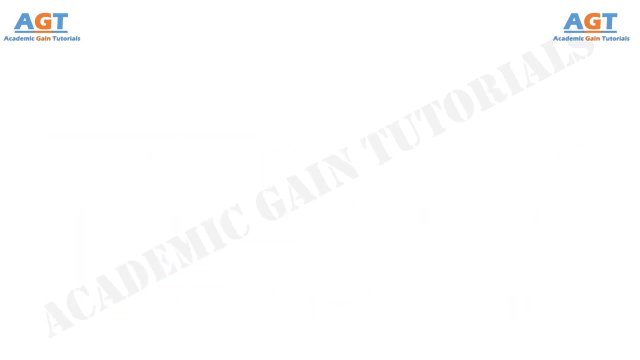 Simply saying: ergonomics is a way of working smarter, not harder, by designing tools, equipment, workstations and tasks that allow a job to fit the worker and not by fitting the worker to the job. Now that we have discussed and defined the concepts about human factors, engineering and ergonomics, let's look in details about what ergonomics is.